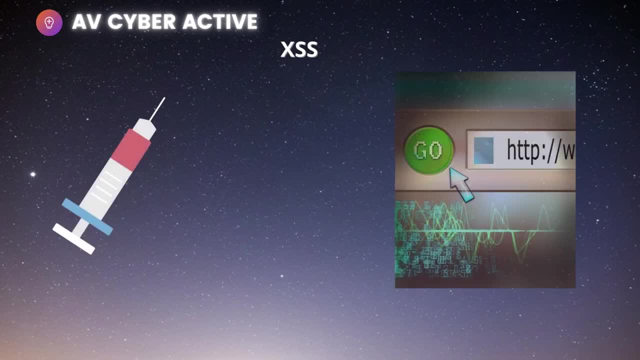 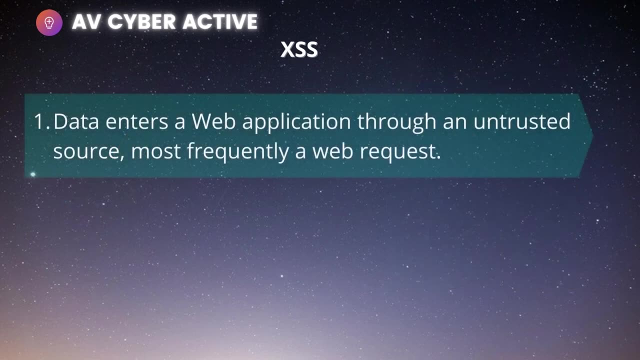 scripting. at the very core, It's injecting a script. So when does that cross-site scripting happen? It happens when a data enters a web application through an untrusted source and most probably or most frequently, it gets in through a web request. Secondly, the data that is included in the dynamic content that is sent to the web user. 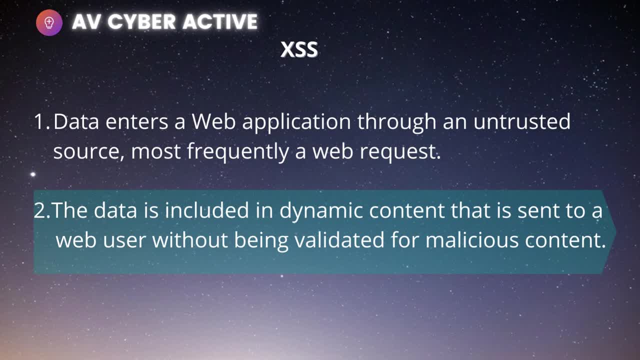 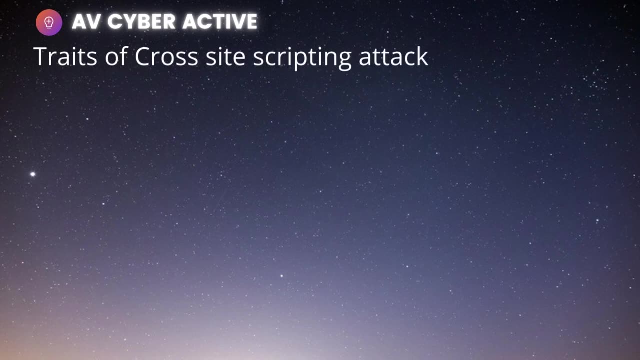 is not even getting validated for malicious content. So if a script is included with the tag or the input in the web request, that gets executed on the web application side. Also, what are the traits or what are the key features of a cross-site scripting? 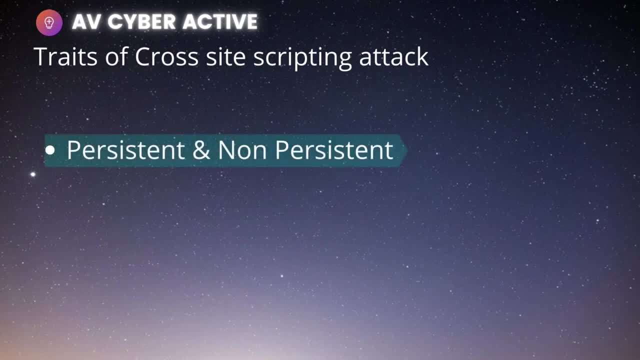 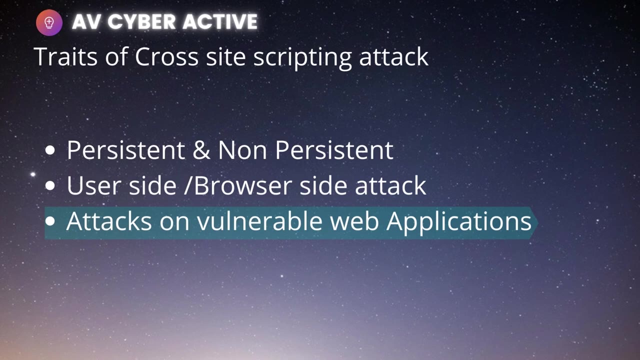 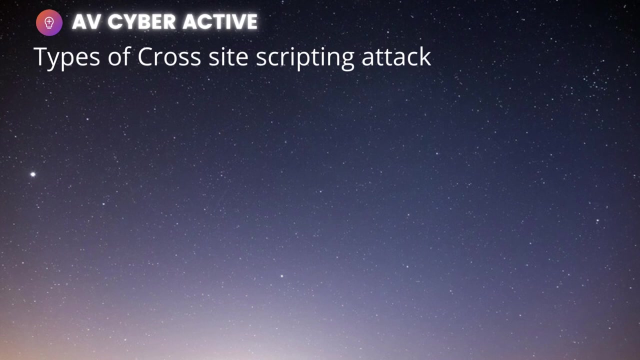 It's either persistent or it's either non-persistent. It's also a user side or you can say a browser side attack, And it always attacks the vulnerable web applications to inject the code or store its code. Next, what are the types of cross-site scripting? The most common ones are these three: 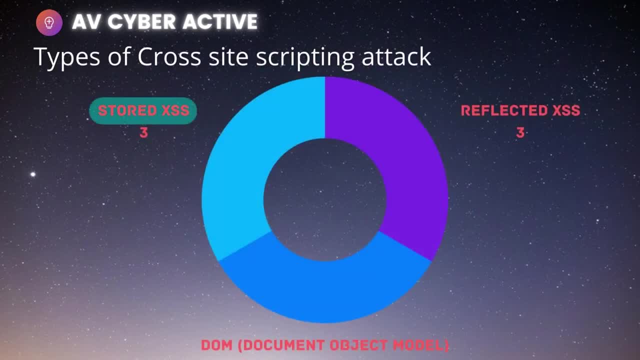 which is stored, cross-site scripting, which is our persistent, reflected cross-site scripting, which is non-persistent, and DOM cross-site scripting, which means document model, object model. In this session, we're not going to discuss all three of them. It would need a. 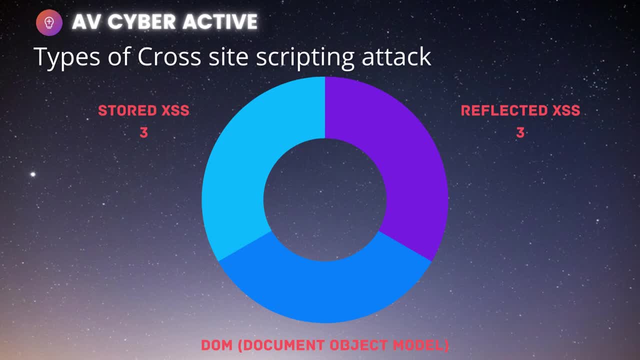 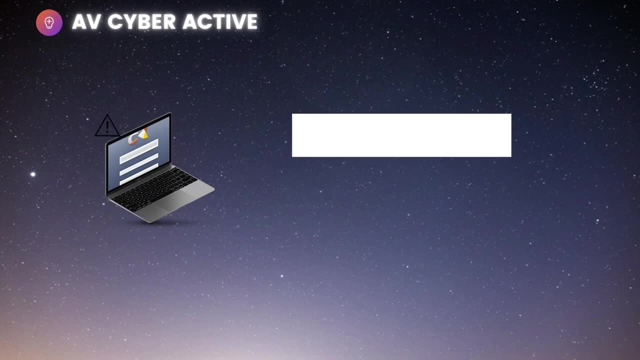 dedicated video for each one of them to explain, but I'll certainly go through the reflected cross-site scripting, which is the non-persistent version of it Now. reflected cross-site scripting, XSS. What is it that comes to your mind when you think of? 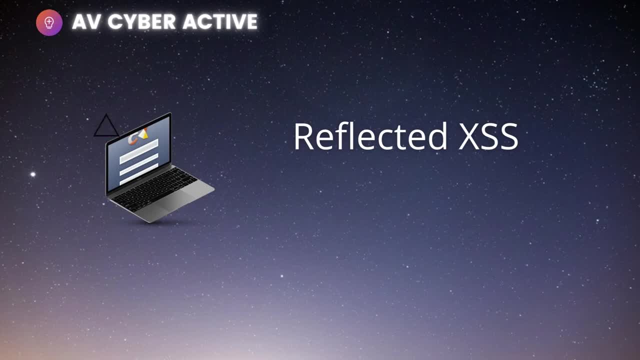 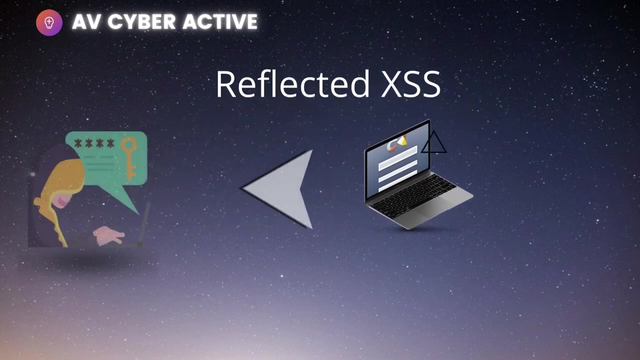 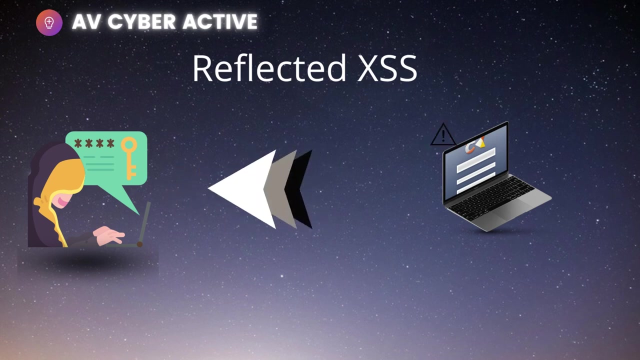 reflected, XSS or reflection reflected. You think of something getting reflected back. You look at the mirror. your image of yours is reflecting back at you. So something similar is also happening here. You see that the vector is trying to reflect some information back to the victim's. 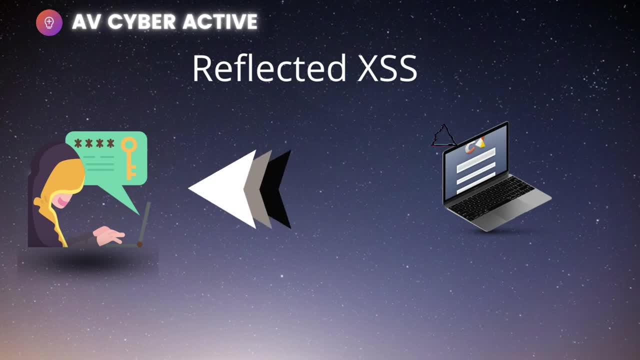 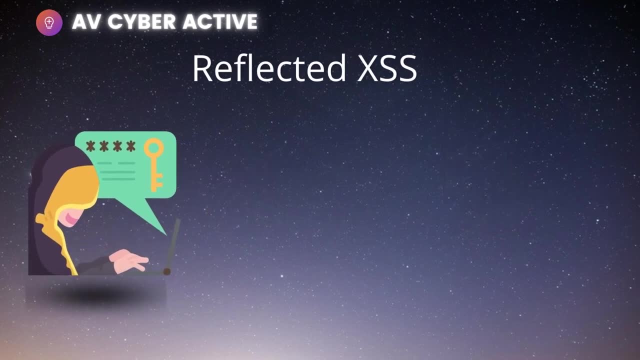 browser so that its motive is getting fulfilled. That's what's happening here. Now let's bring up our bad guy or the perpetrator. So the script is activated through a link which sends a request to a website with the vulnerability that enables the execution of the malicious. 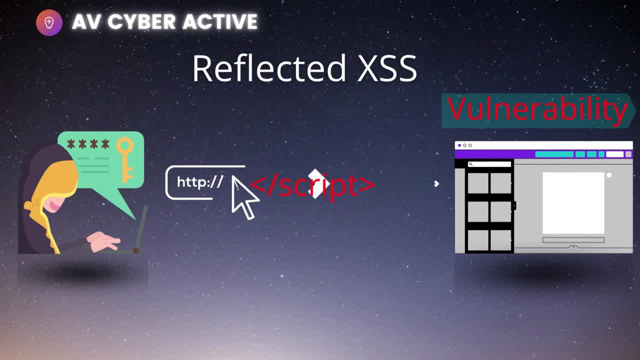 script. This vulnerability is a result of the incoming request. if not properly sanitized or checked during the development of the web application, allows the manipulation of the web app functions and the malicious script gets activated. Then the intended information gets reflected back, because it is of course. 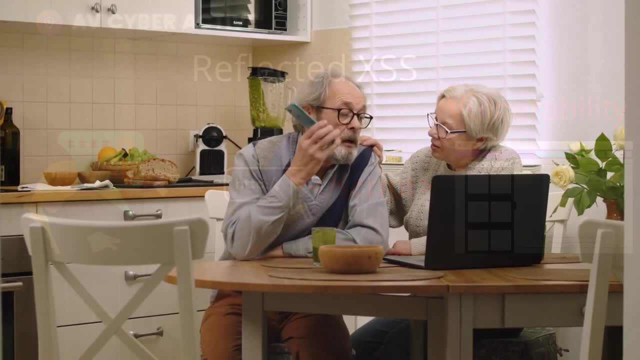 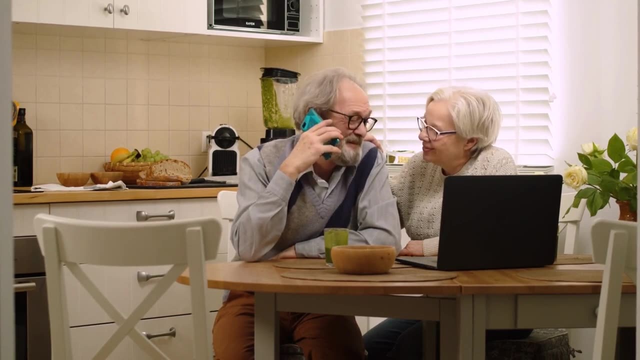 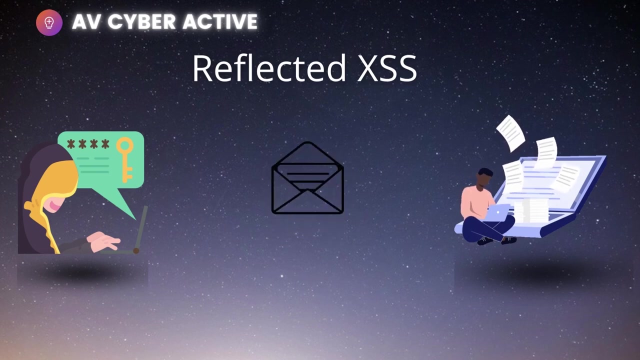 vulnerable and is now sent back to the perpetrator. Now you would think, why would the user even click on the link? And this is where the user is lured into social engineering. So the bad actor would distribute the malicious link to the perpetrator, typically in an email or a very lucrative looking 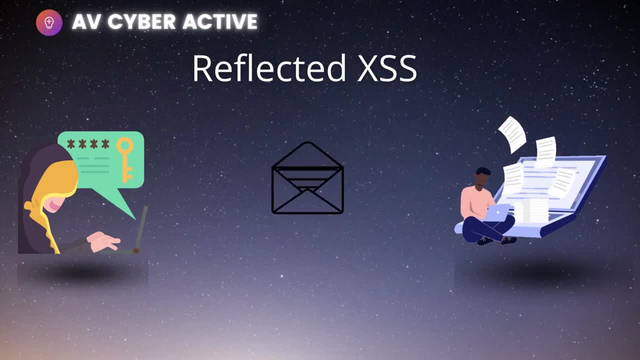 email or website. The link is embedded or an anchor text provokes the user to click on the link. Click on it, which then initiates the cross site script request to the exploited or the vulnerable website, reflecting the attack back to the user. 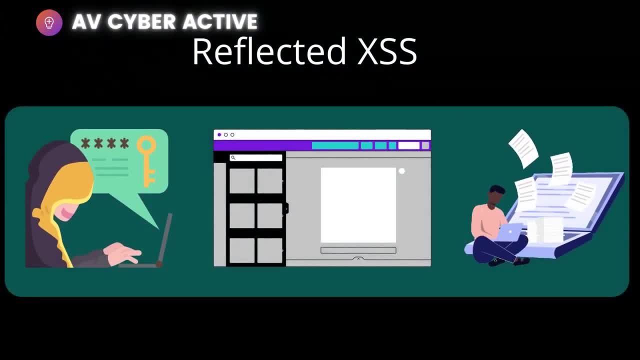 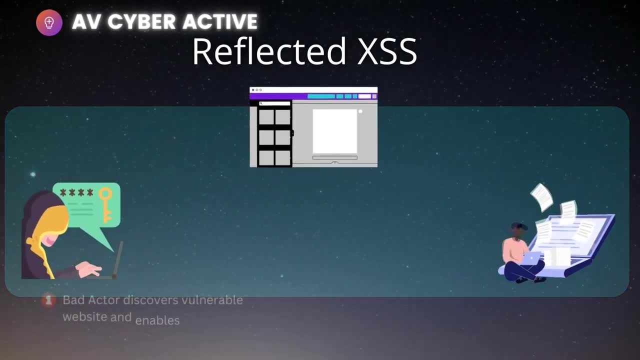 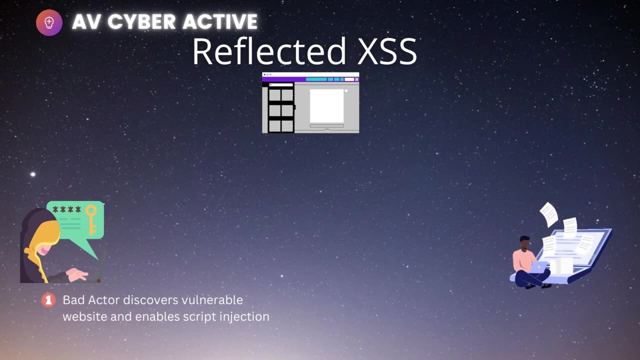 Now there are quite a few things happening out here. Okay, let's try to understand that. So we got a perpetrator, the victim and the vulnerable website. Step one: the perpetrator will discover the website having the vulnerability and will enable the scripts for injection. 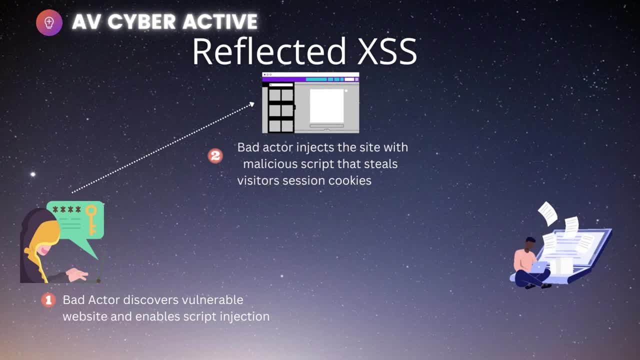 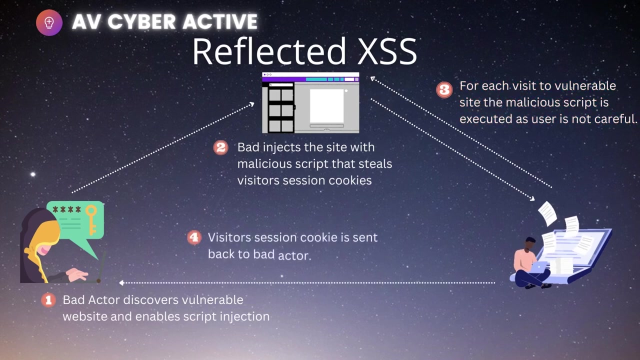 step 2: perpetrator will then try to inject the website with the malicious script that steals the visitors you know, cookie sessions or any confidential information. step 3: the most dangerous part: for each visit, the malicious script is reflected back at the victim and the script gets activated then, as the perpetrator wanted, the. at step four, the. 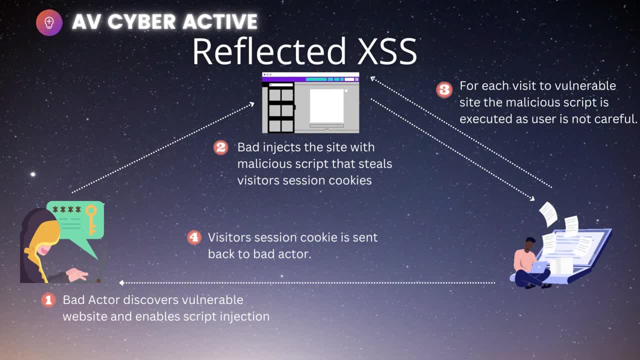 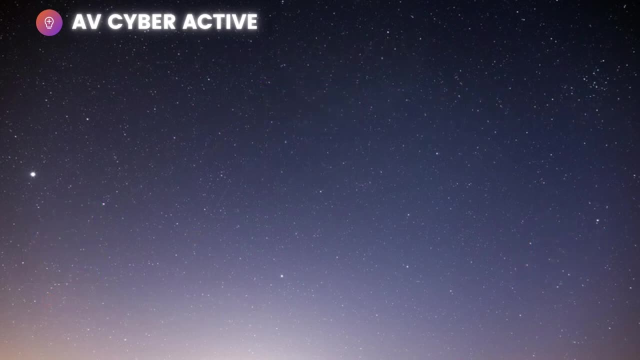 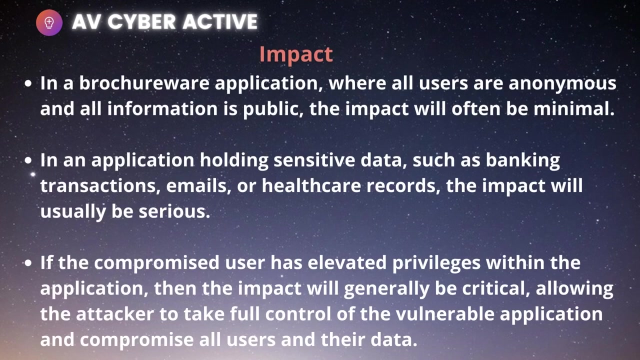 visitor session cookie. all the uh secret information is then sent back to the perpetrator so that the bad actor can now use it to its advantage. now you must be sitting out there thinking, how does that impact me? fine, crosshead scripting. well you, here's what you should consider. the actual impact of a cross-site scripting attack is generally. 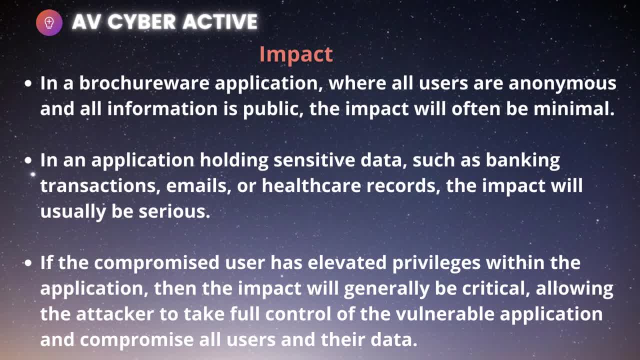 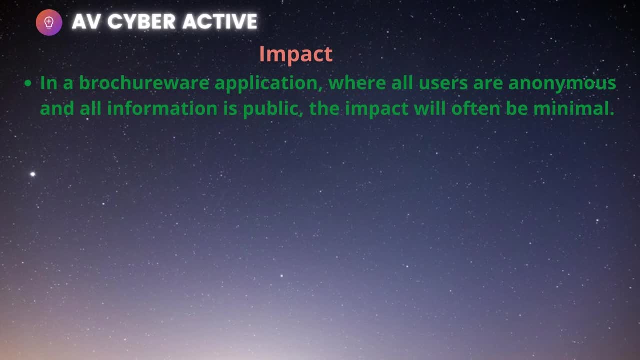 dependent on the nature of application and its functionality on the data. it also depends on the status of the compromised user. i'll take three examples. if it's a regular, just an informational or a brochure aware information on application- a web application, in this case, where all of your 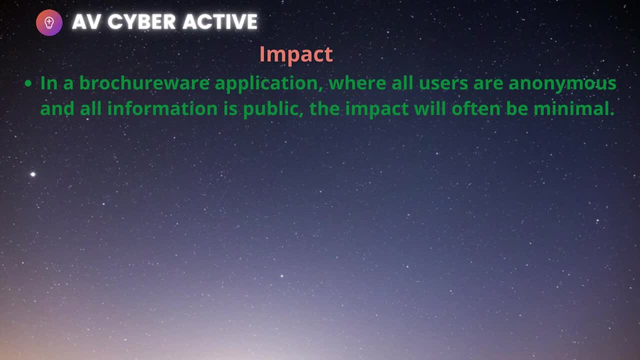 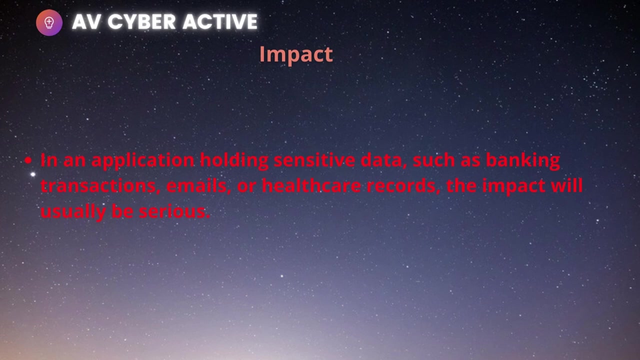 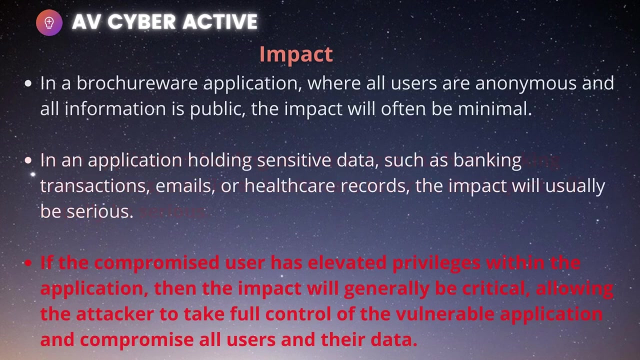 users are just anonymous and the information is purely public, the impact will obviously be very minimal. but if an application is hold holding sensitive data, such as banking transactions, your emails, your health care records, then the impact is going to be significantly more and very serious. third, if the compromised user 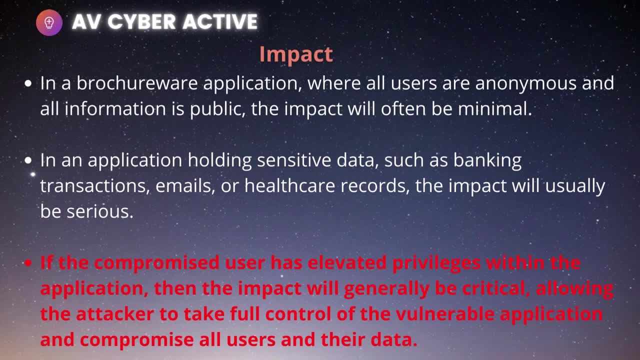 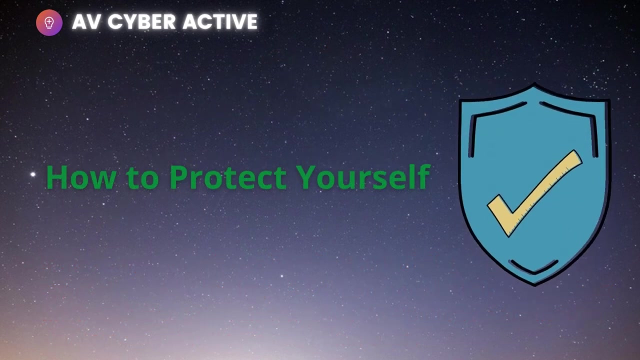 or the victim has, you know, elevated the privileges with the application, then the impact will be very critical, allowing the attacker to take full control of your, of the vulnerable application and compromise probably all the users and their data. how about that? now that you know the cross-site scripting and how it works and how dangerous it is, what can you do to protect? 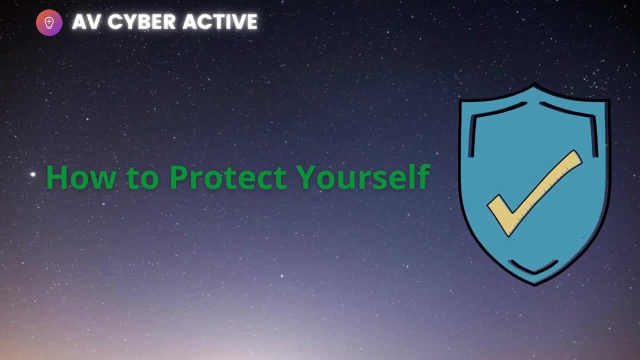 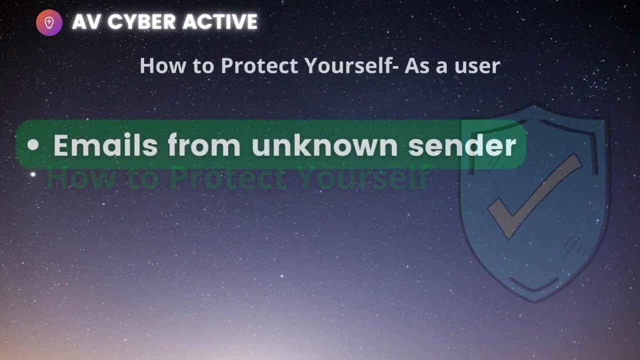 yourself. i'll give you two perspectives: one from a user's perspective, another one from a developer's perspective. as a user, do not click on links on that come via email from unknown senders. okay, those lucrative emails, those lotteries that you went from a nigerian king, those are not happening. 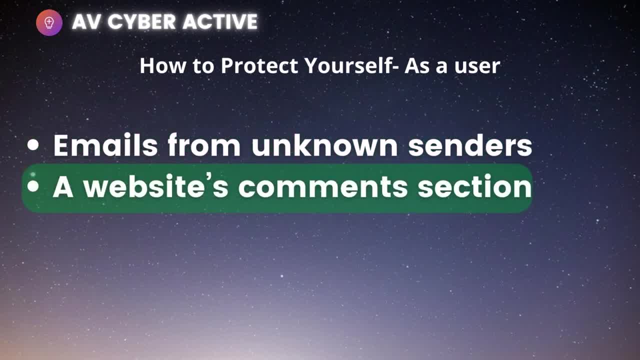 everything is fake. do not click on the link on a website and click on the link on the website to get to the website's comment section. okay, if you go to a shady website, if you see there's a lucrative link to win or something and you would have to contact somebody else, just just don't con comment on those. 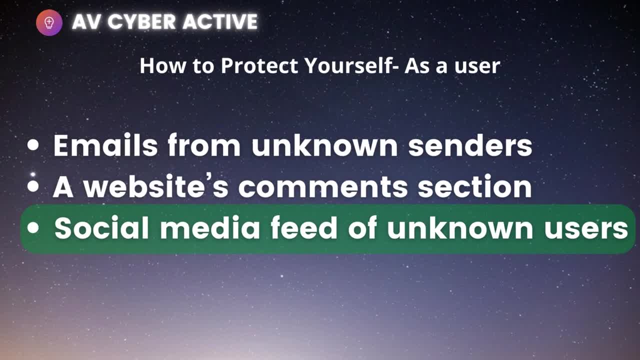 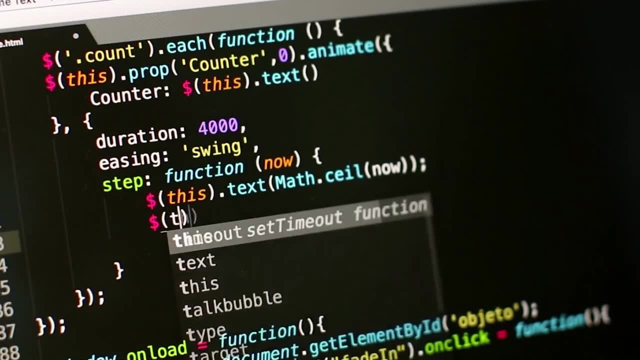 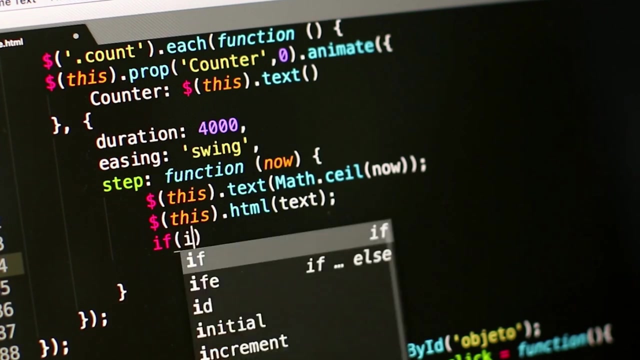 links. so, and the last one, social media feed of unknown users. okay from developers perspective. well, preventing cross-site scripting is trivial in some cases, but much harder depending on the complexity of the application and the ways it handles the user. controllable data, but, in general, effectively preventing cross-site scripting vulnerabilities. 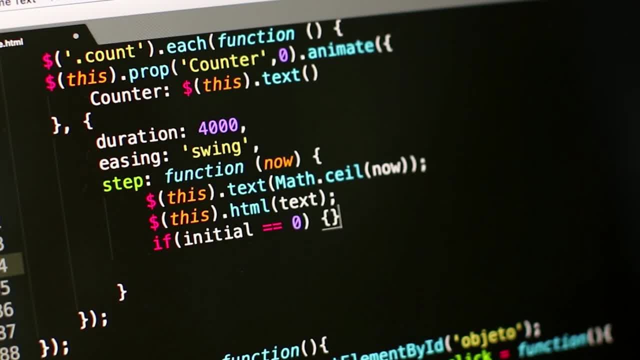 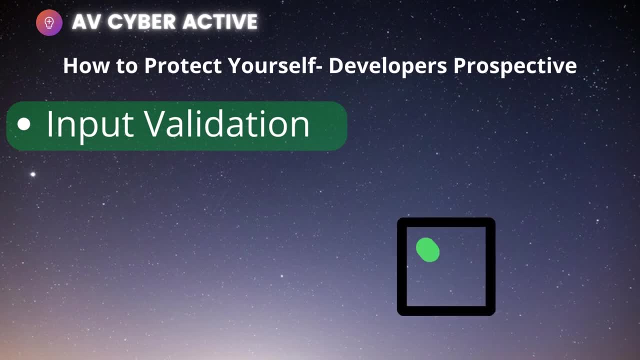 is like lead is likely to involve a combination of the few measures. that which i'm going to talk about, first of all, input validation filter: input on arrival, at the point where the user is user input is being received. this field: keep your filter as strict as possible. 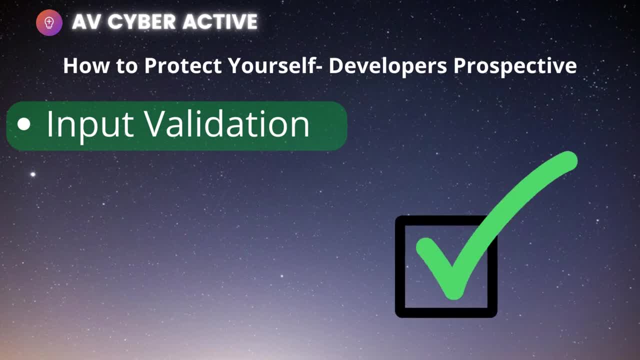 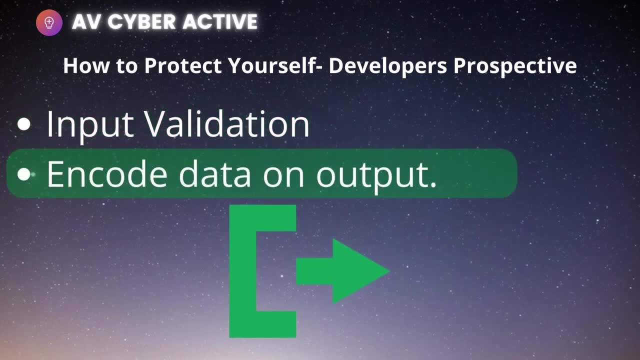 and nothing unexpected should be entered. second, encode data at output. what does that mean? so, at the point where the user controllable data is output in the http responses, and code the output to prevent it from interpreted as an active content. so, but so depending on the output context, this might require applying. 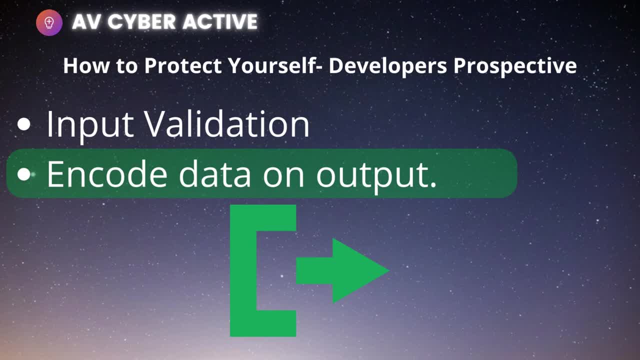 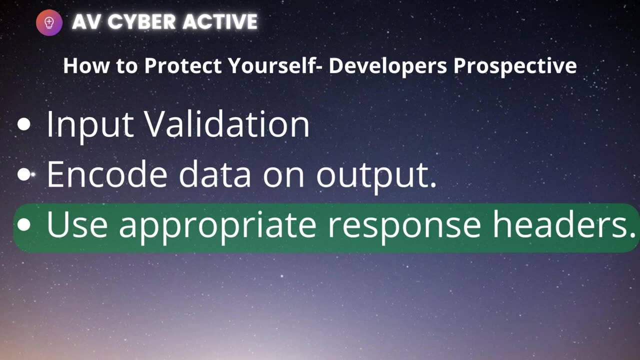 combinations of html, url, javascript and css encodings. next one: use appropriate response headers to prevent cross-site scripting and http responses that aren't, you know, intended to contain any- uh, it's html or java. you can use the content type options in the headers to ensure that the browsers. 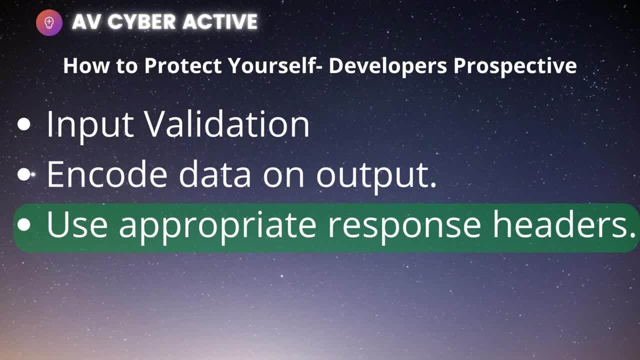 do not interpret those responses, uh and or browsers interpret the responses in a way you intended, intended it to be designed. and the last one: content security policies as the last line of defense. what you can do is you can use a csp contract, you can use Cloud Interface, which is basically a standard.